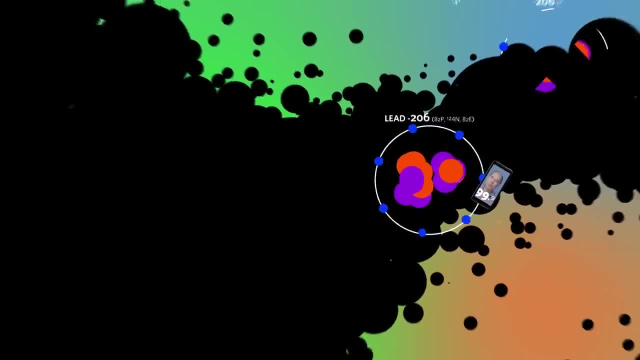 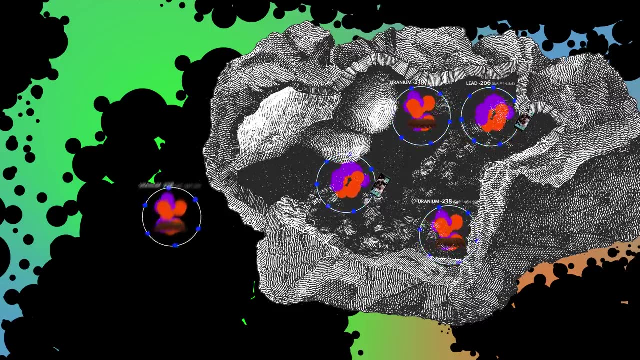 isotope is the decay of the parent. You also need a rock that behaves a bit like a sealed time capsule, preventing daughter isotopes from leaving and keeping new parent isotopes from wandering. in That way, if you end up with half-daughter and half-parent isotopes, you know. 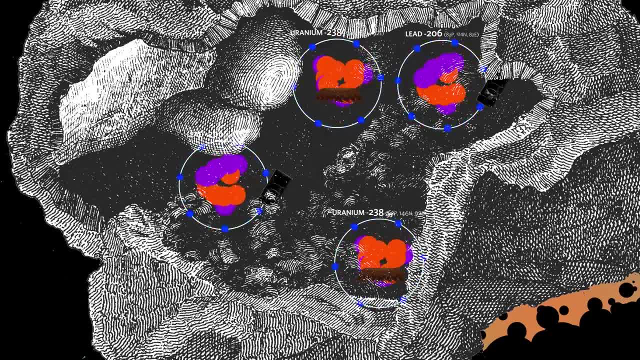 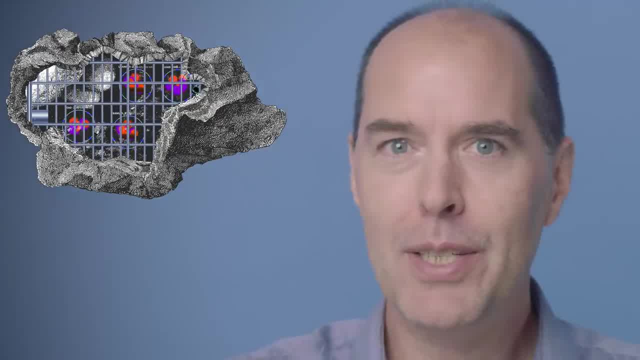 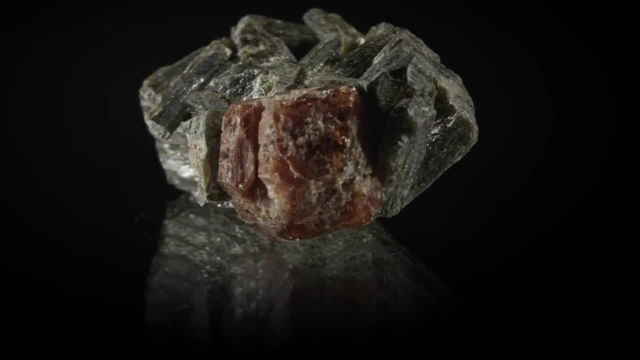 that one half-life has gone by since the rock kept everything locked into the same place. Certain minerals form a tinker toy-like cage around any larger isotopes. This locks everything in place and makes for an excellent time capsule. Zircon crystals, for example, can trap atoms of radioactive. 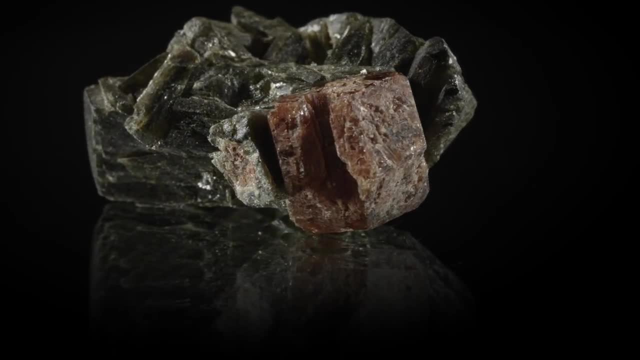 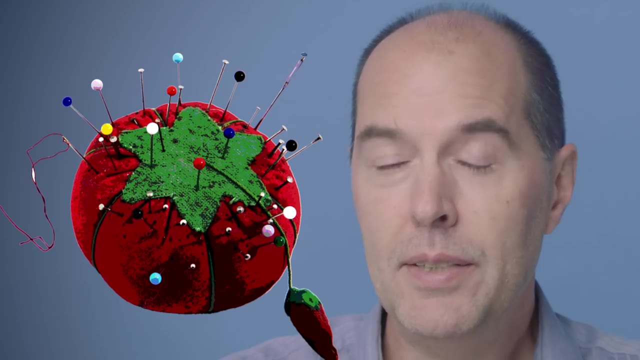 uranium inside the rock. Zircon crystals, for example, can trap atoms of radioactive uranium inside them, as well as its daughter isotope, lead. So measure the proportion of uranium to lead in a zircon crystal and you can figure out when it must have formed. Take this tiny. 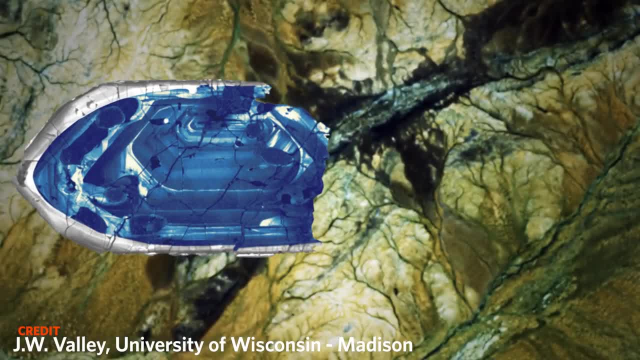 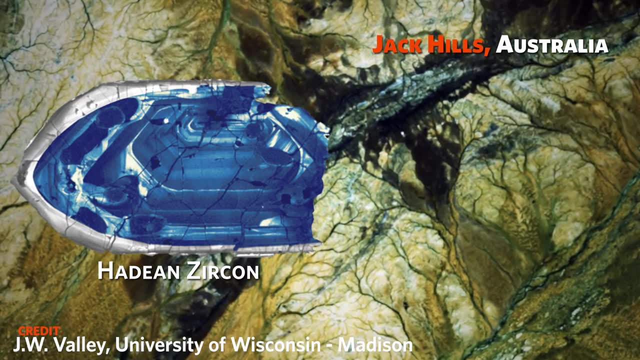 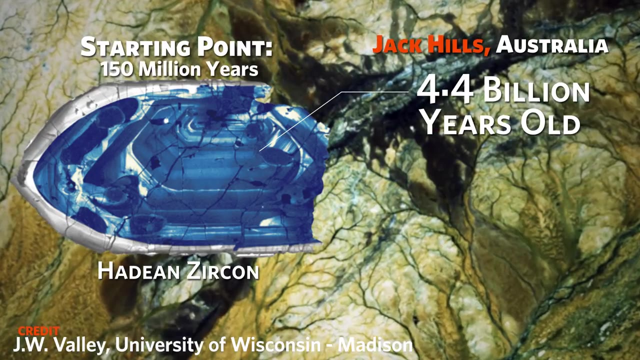 zircon, for example, which would fit comfortably on the head of a pin. Believe it or not, this tiny zircon, which comes from Western Australia, is the oldest piece of Earth we've ever found. It's an absolutely mind-blowing 4.4 billion years old and comes from when the Earth was only 150 million. years after its formation. Zircon crystals, for example, can trap atoms of radioactive uranium inside the rock. Zircon crystals, for example, can trap atoms of radioactive uranium inside the rock. Zircon crystals, for example, can trap atoms of radioactive uranium inside the rock. 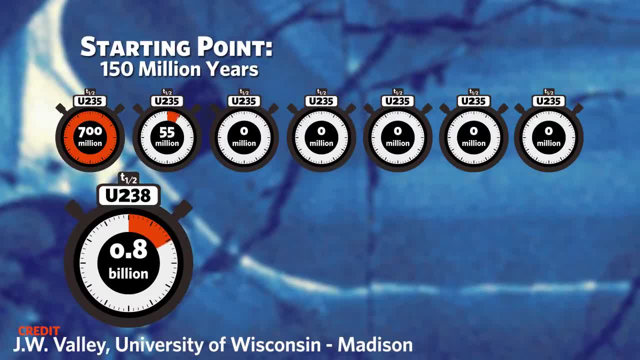 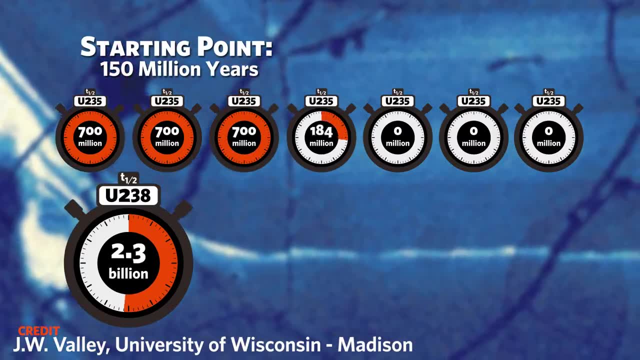 The zircon was dated using two different isotopes of uranium: uranium-235 and uranium-238.. This provided a built-in cross-check, as you had two different clocks keeping time within the crystal. Whichever clock you look at, they give the same result: The uranium's been trapped in. 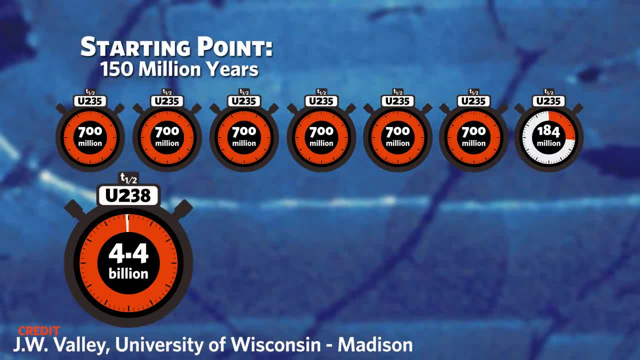 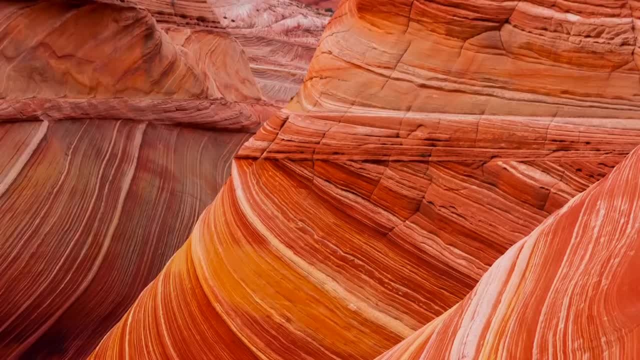 that zircon, since it formed 4.4 billion years ago. Most dating techniques only work with certain types of rock. You can tell when lava erupted, for example, but can't figure out when sandstone formed. That's because the sandstone doesn't trap isotopes in the 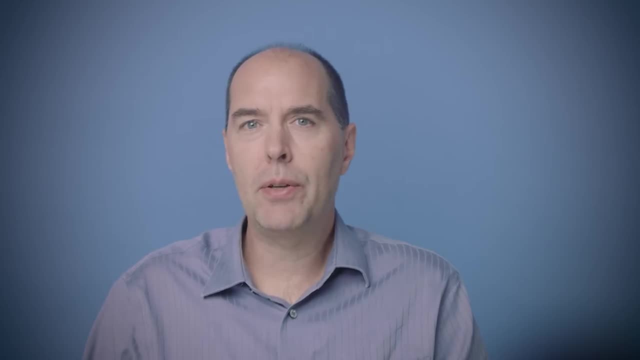 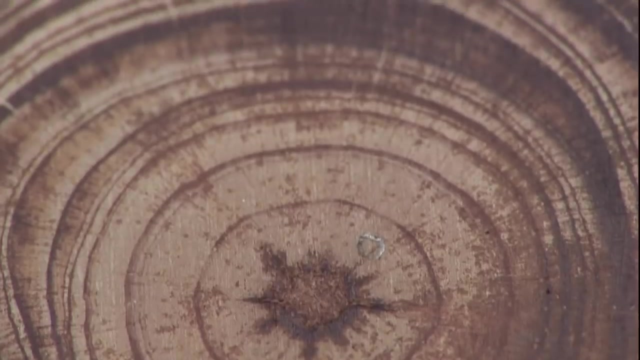 tinker-toy-like cages that we mentioned earlier, Because there are other ways to tell how old things are in the world. we can compare those results with radiometric dating and show that they match. Trees, for example, put down a new ring each year. they grow and you can count.